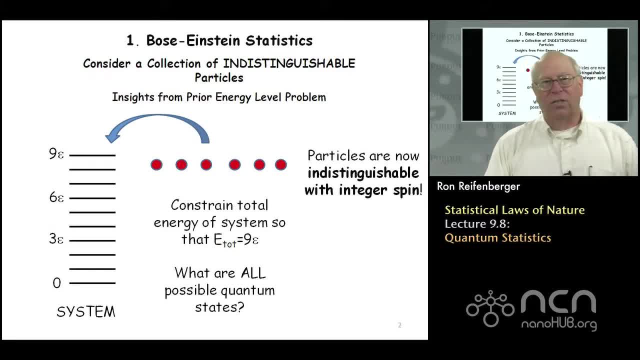 each state that was possible. So in this lecture, I think it would be very helpful if you printed out this slide, this table- it's actually given to you on the website- because we're going to be referring back to it and we're going to try. 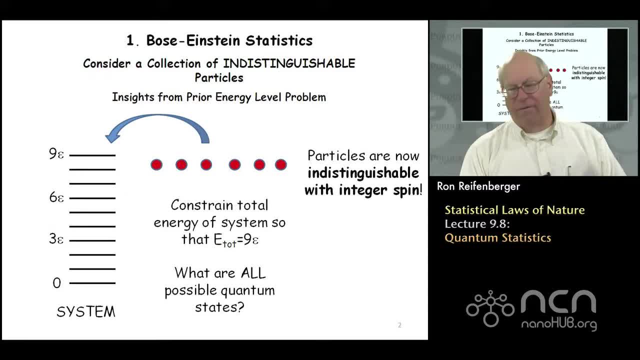 to understand how this table is modified when we make the particles indistinguishable. So what we're going to do now is we're going to remove the color from the particles. before, each particle was colored a different way so we could distinguish them. Now we're going to make all the particles the 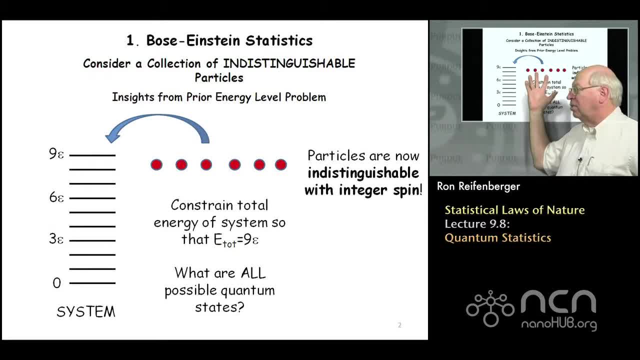 same color and we're going to say we take these 6 particles, we put them in this system and we're going to constrain the total energy to be equal to 9 epsilon. That's the same constraint that we used when we considered this, when we 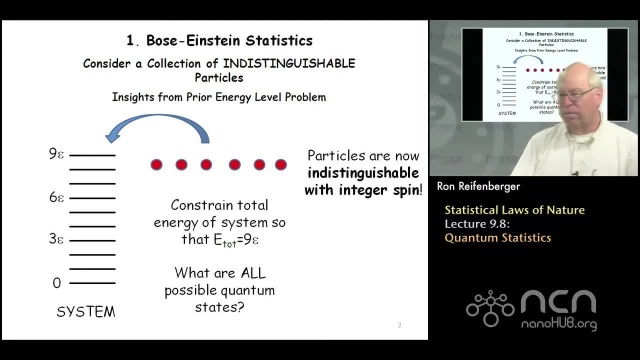 generated this table, So we're trying to compare and contrast the indistinguishable case with the classical distinguishable case that we generated when we first wrote down this table- So that's the plan. and when we're finished with the Bose particles, so these particles have zero spin or integer spin. 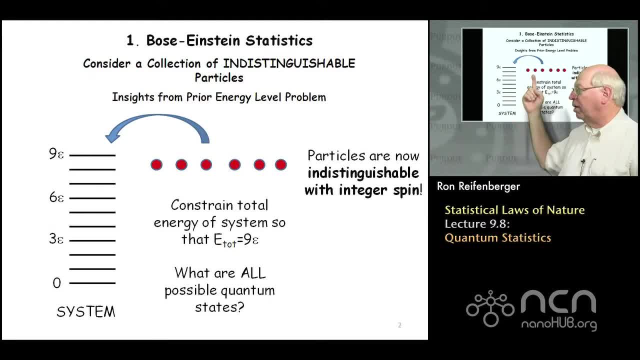 when we're finished with them, we'll also consider particles that are indistinguishable but have spin one half, and we'll talk about the difference in the way the particles can occupy these states. that's related to the quantum nature of the particles. So what we have 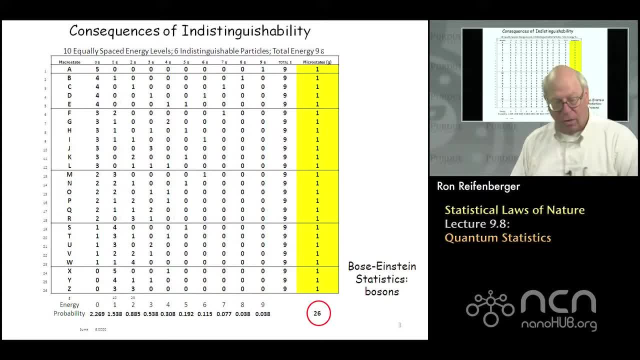 to do is we basically have to go back and reevaluate this table and we have to ask the question: what happens when you remove, when you make each particle indistinguishable one from another? Well, since the total energy of the system is the same, 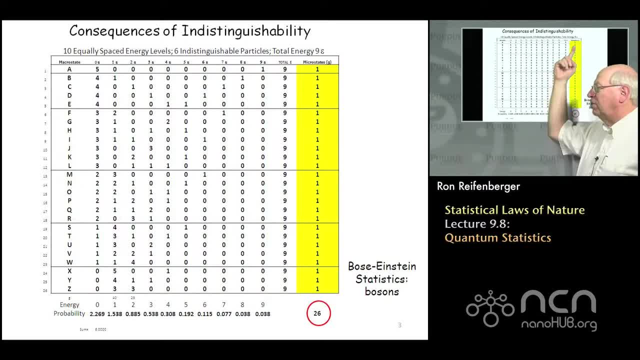 the total energy of the system is this: 9 epsilon. this column doesn't change. and all these different so-called macrostates. there are 26 of them, labeled by the letters in the alphabet. so you go from A to Z. all those states remain the. 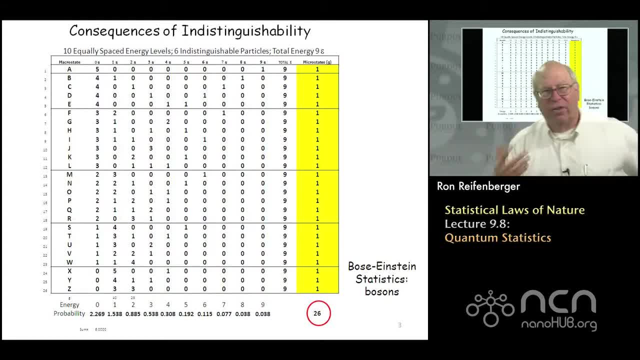 same. The thing that happens is because the particles are indistinguishable. now there's only one way to achieve each possible macrostate. So these degeneracies that were listed in this previous table, which took a fair amount of thought, but they're not going to change in the 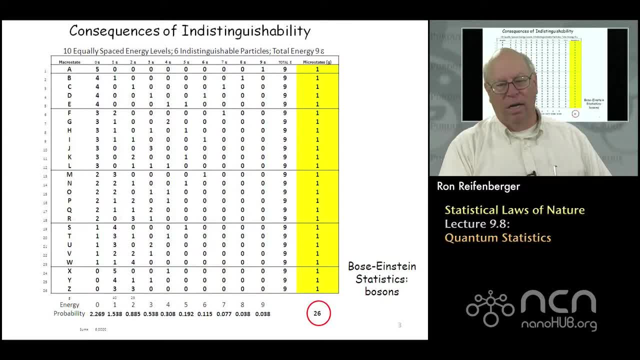 future. There's a lot of thought to generate those degeneracies. they completely disappear and we now have a total of 26 possible states. When the particles were distinguishable, you'll remember that we had 2002 possible microstates. now we've only got 26. And that completely changes. 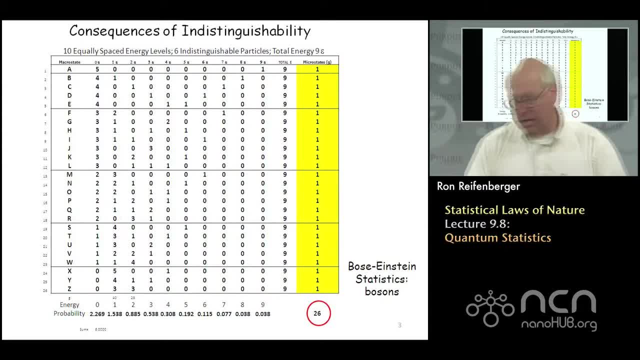 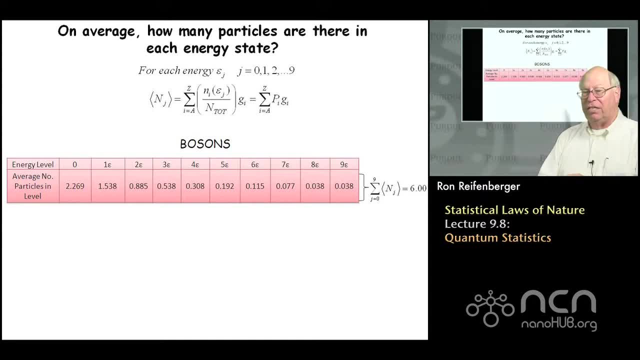 the statistics right. That completely changes the statistics. To illustrate that, I'd like to just ask the question: on average, how many particles are there? How many are there in each energy state, now that the particles are indistinguishable one from another? 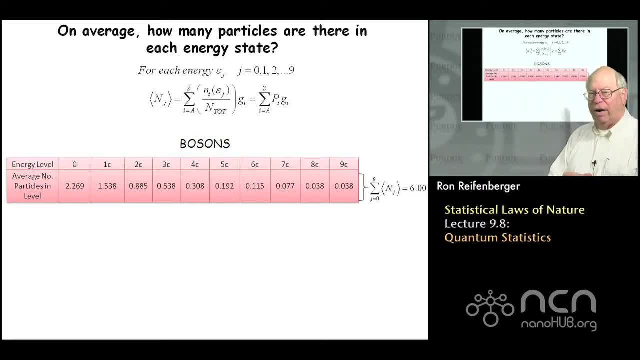 Well, we're going to follow exactly the same program we did when we calculated the case for the distinguishable particles. The average number of particles in the energy state J is basically going to be the sum over all the states. there's 26 different states. 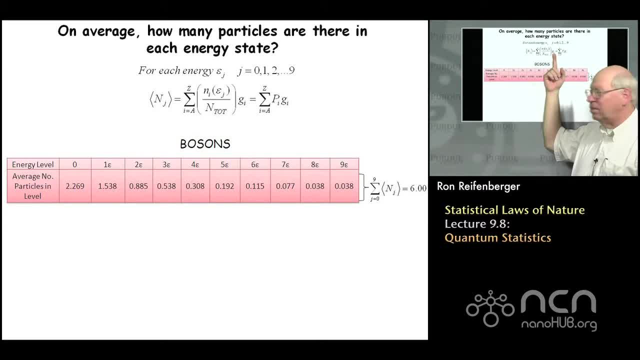 The degeneracy of each state has to be included. we have to calculate the G sub I quantity. we have to calculate from this table. we have to estimate the total number of particles in a particular state, J, and we have to divide that by the total number of particles which in 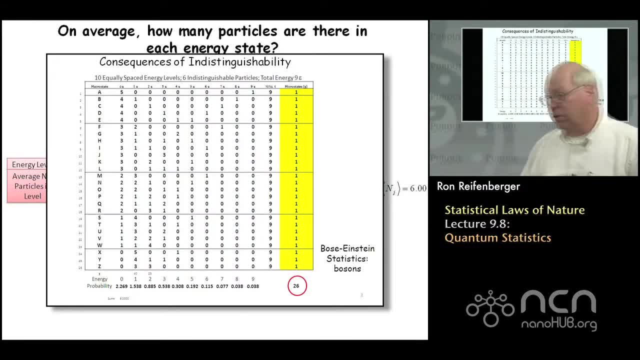 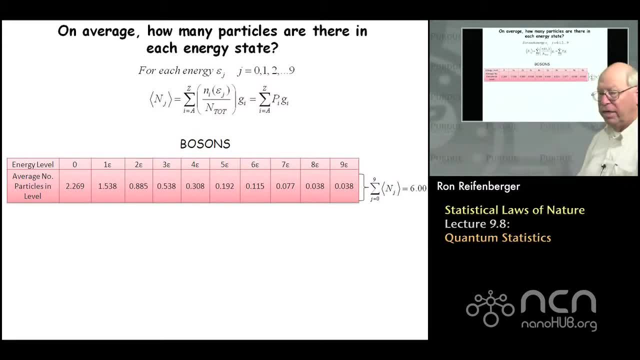 this case is 6.. So what we have to do is we have to use this table with these degeneracies to calculate these average numbers of particles, And so I just list the results of this calculation. you can go back and check it for one case. 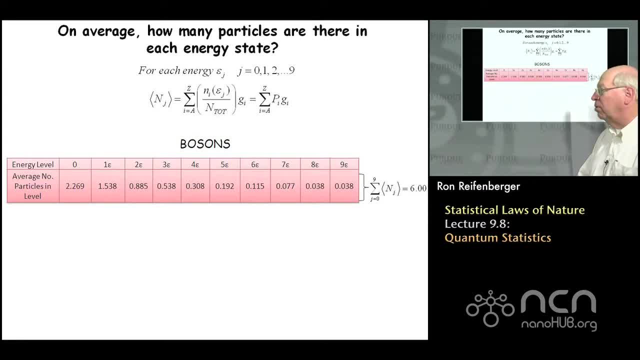 it's a lot easier now that the particles are distinguishable, and if you run the numbers yourself, I'm sure you'll agree with the results that I provide. I sort of think these numbers are correct, because I don't want to go up. I ought to get 6,. 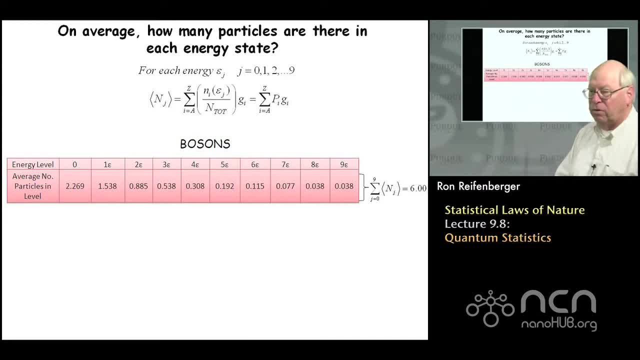 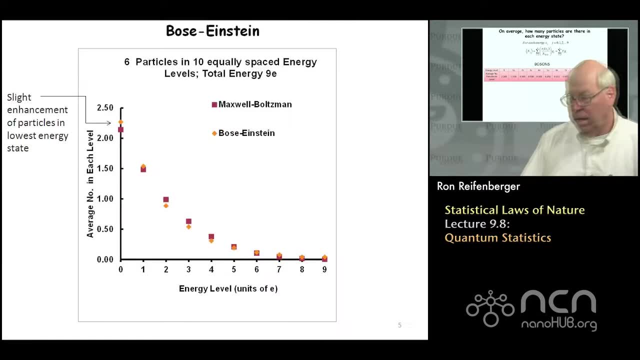 and I do because 6 is the total number of particles available in the system. These just tell you on average how many particles will be in each energy level. It's very instructive actually to plot this new distribution. This new distribution is named after the Bose-Einstein theoretical distribution. 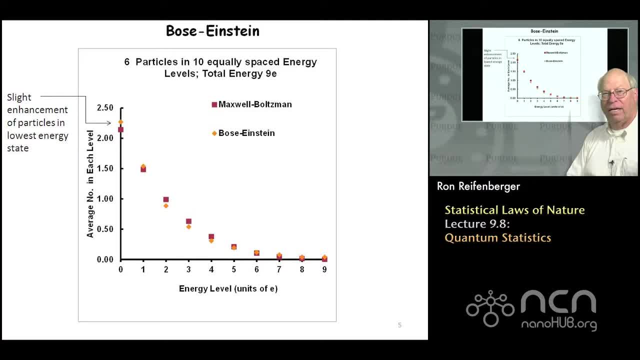 that was derived independently by both Bose and Einstein back in the 1920s, And it's very interesting to compare the average particle number in each energy level to the results that we obtained from the Maxwell-Boltzmann discussion that was based on this. 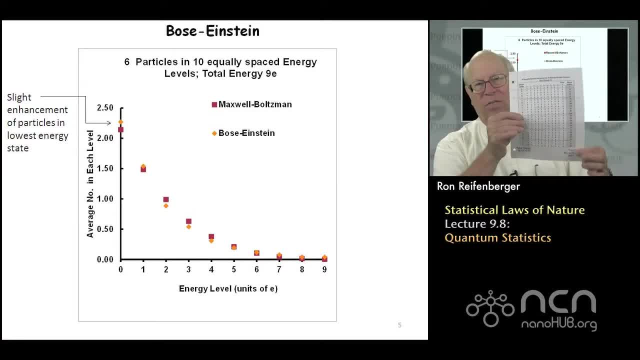 rather large table with these 2,002 multiplicity levels And that comparison is made in this graph. I just basically am plotting the number of particles in each energy level. I just basically am plotting the occupation number. the average number of particles in each energy level is a function of energy. 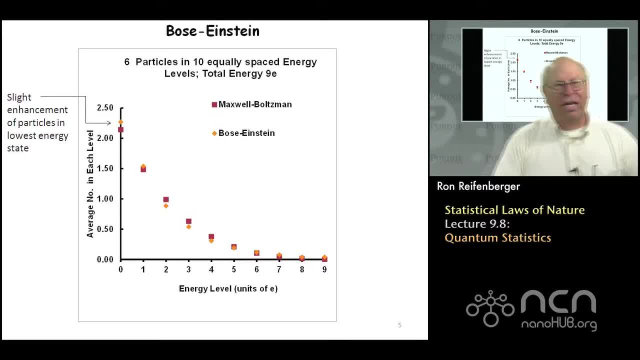 You can see the Bose-Einstein number compared to the Maxwell-Boltzmann number And they're slightly different even for 6 particles. You can start to see a slight difference in the 2 distributions. This is related to the fact that the Bose-Einstein 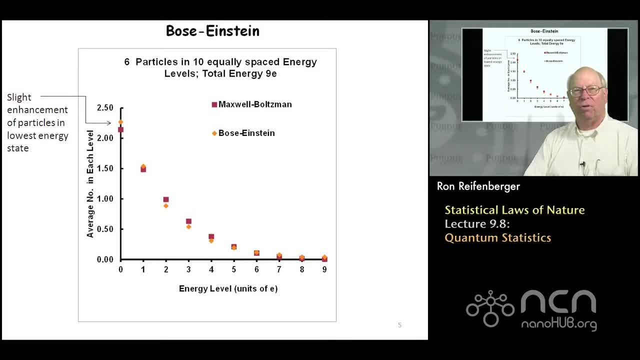 particles are now strictly quantum mechanical and they are indistinguishable. Once they become indistinguishable, the multiplicity of these allowed energy levels drastically changes. When you change that multiplicity, you change the number of particles in each energy level And, in particular, what I 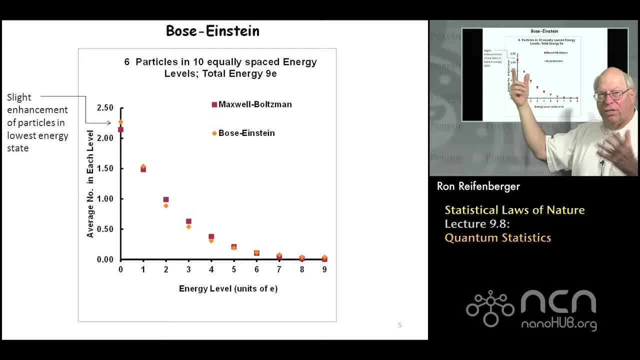 like to call your attention to is the fact that if you have 6 particles, which is by no means a large number of particles, the Bose-Einstein distribution at the lowest energy level, which is the zero value, is actually slightly enhanced over the classical Maxwell-Boltzmann distribution. 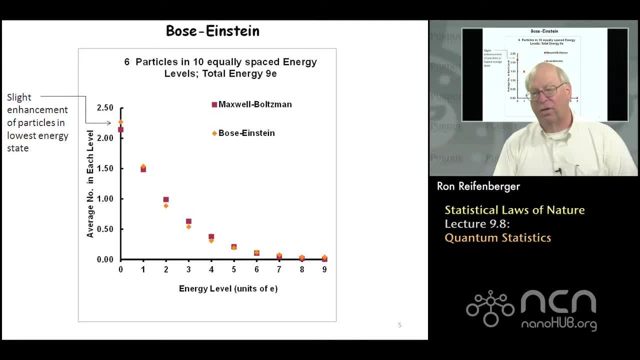 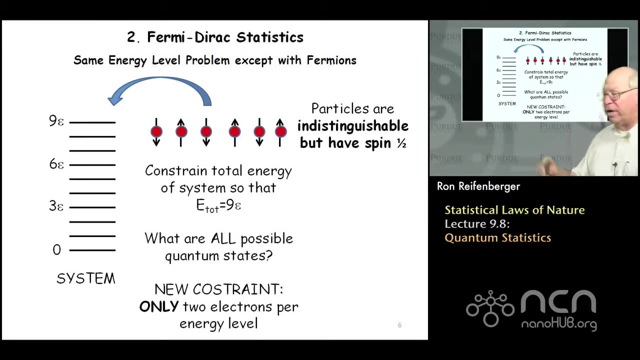 And this slight enhancement is going to be a characteristic signature of Bose-Einstein statistics, as we'll describe as the lecture unfolds. We can follow the same program for Fermi particles, right? So the Fermi particles now are going to have a spin one-half. so let's pretend. 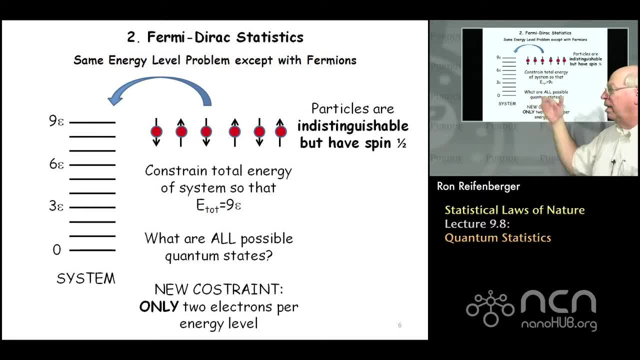 these are non-interacting electrons And they are governed by Fermi-Dirac statistics. Fermi-Dirac statistics are named after Fermi and Dirac, who derived these statistics independently again back in the 1920s. We're going to consider. 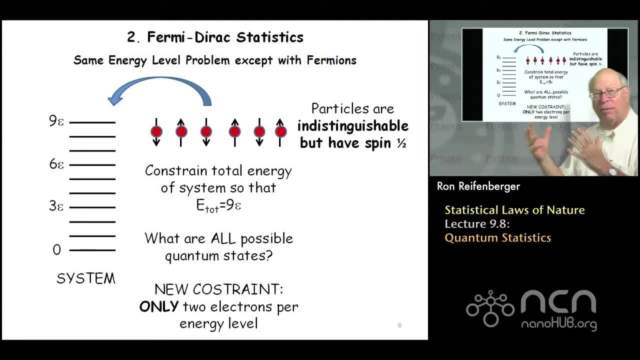 the exact same system that we've considered for the Bose particles. We're going to now have 6 indistinguishable particles. They have spin one-half, so they're fermions. We're going to give these particles collectively a total of 9 energy units and we're 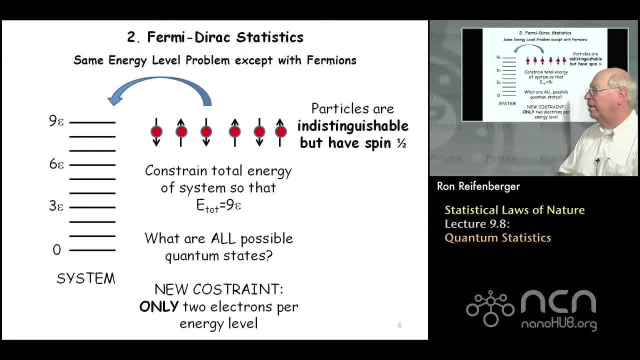 going to ask what is the distribution of these particles in this 10 energy level system And we're going to compare that to what we got in classically, because we're going to try to understand what are the differences that are imposed by the constraint that these particles are indistinguishable. 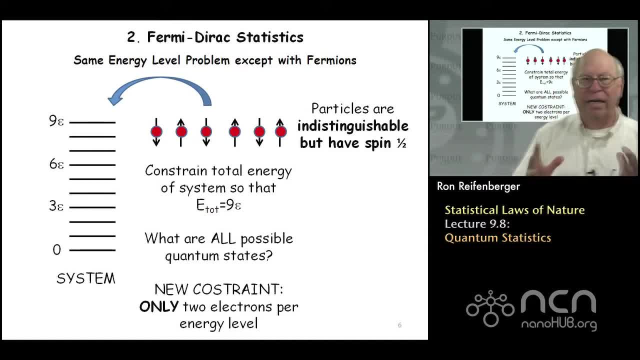 and have spin one-half. Well, the new constraint is that these Fermi particles, you can only put two particles in the same quantum state, So the difference in quantum number has to come from the difference in the spin of the particles, and that just basically means that you only can get. 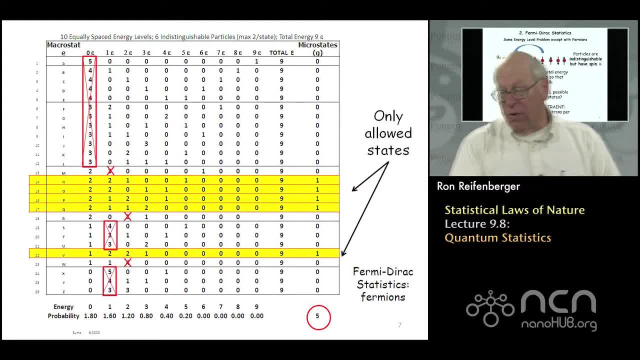 two electrons per energy level. Well, that has a drastic consequence on our table of possible states of the system, because what we can do is we can look through this table and any time we have an energy level that has more than two particles in it. 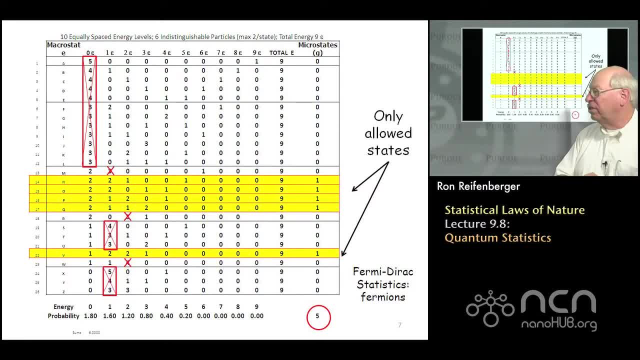 that energy level or that state is going to be forbidden. So, for instance, all these states here which have three, four or five particles in the zero energy state, those are all outlawed. those are no longer possible. Any state that has. 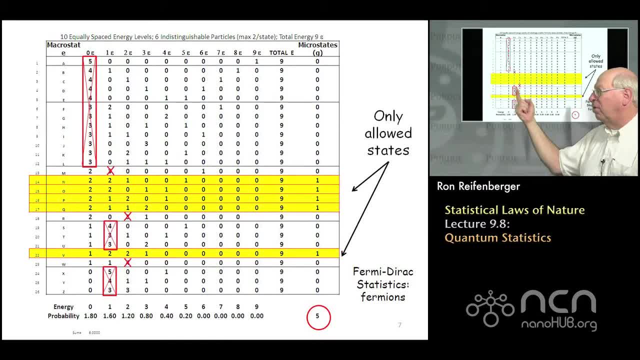 more than two particles in the one energy level is also going to be outlawed. that's no longer possible, And the surprising thing is, if you look at this table carefully, you're going to find that there's only five states that survive this criterion. So these states 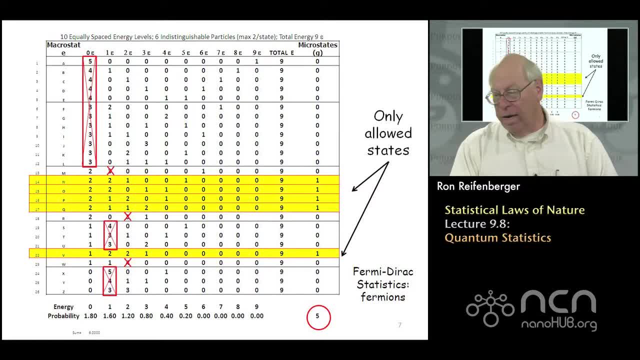 are labeled N, O, P, Q and V in this table. Those are the only states that can satisfy this Pauli exclusion principle. that's based on the spin-one-half nature of the particles. Everything else is excluded. right Now, the number of microstates that we have to 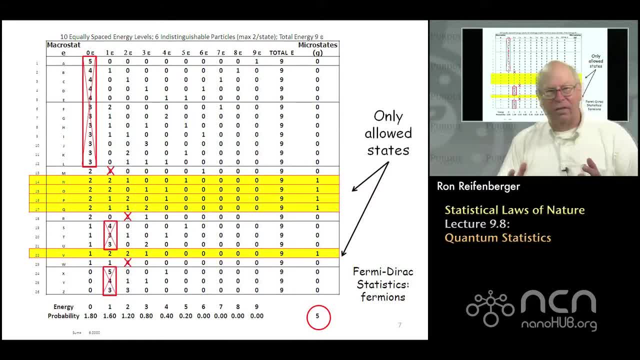 consider is just five, And so we've gone from 2002 for distinguishable particles down to 26 for Bose particles. For Fermi particles, we only have five possible states of the system. We can do the exact same thing we did for the. 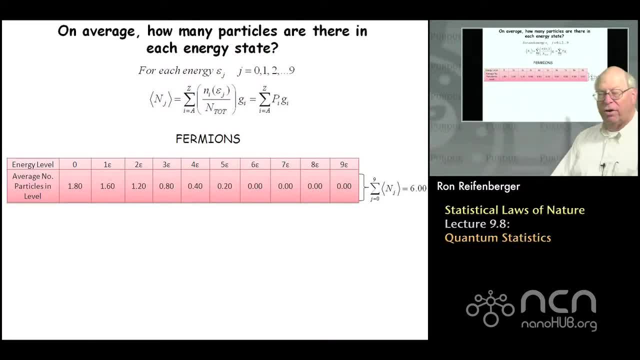 bosons. right, We can ask on average how many particles are in each energy state. We just have to take this definition for the average number of particles And now the calculation is really simple, because instead of summing over all 26 states, there's only going to be 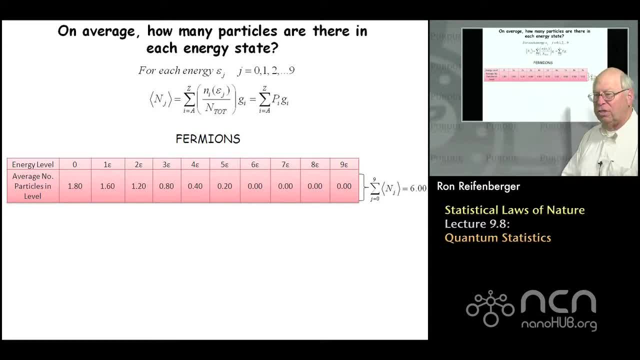 five states that survive, And so this sum is only going to have five energy states associated with it. The degeneracy of each state is again going to be simplified. simplifies the calculation, And these are the results I get. You're welcome to check, right. 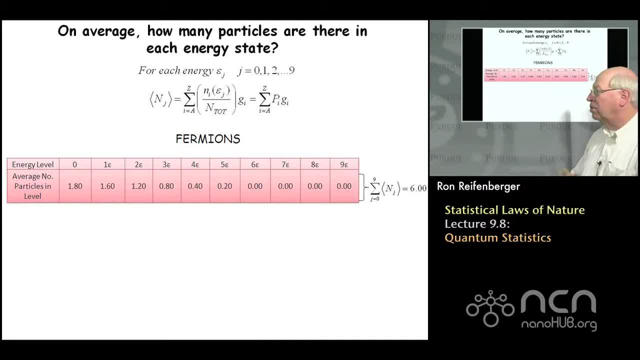 It's pretty simple to double check these numbers. And again, you like to believe that if you add the average number of particles in each energy level, if you add them all up, you're going to get six And in fact if you do that sum, you'll find that. 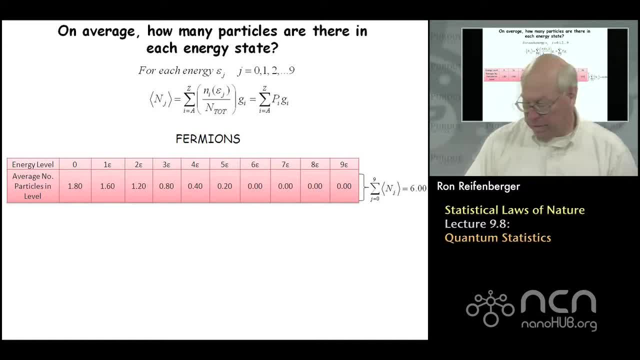 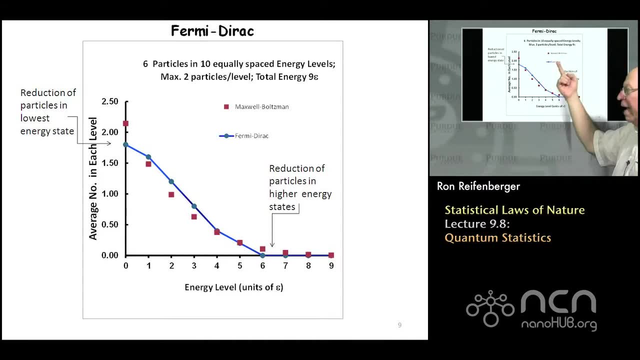 there's only going to be five particles that survive and accounted for in this calculation. It's very useful to compare the results for the Fermi-Dirac particles to the Maxwell-Boltzmann distribution. This is the classic case, right, And what you see is you see that. 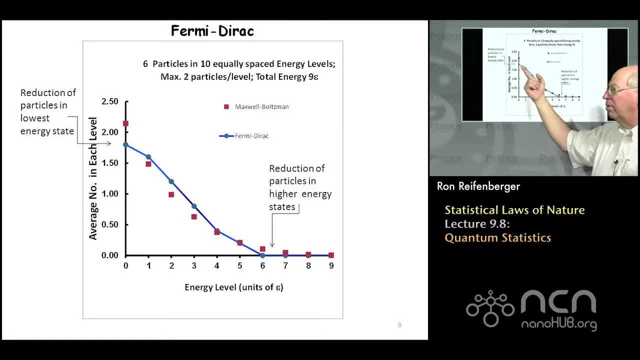 there's actually a reduction of the number of particles in the lowest energy state compared to the classical situation. So, classically, you ended up with, I think, about 2.3 particles in the zero energy level state By imposing this condition on. 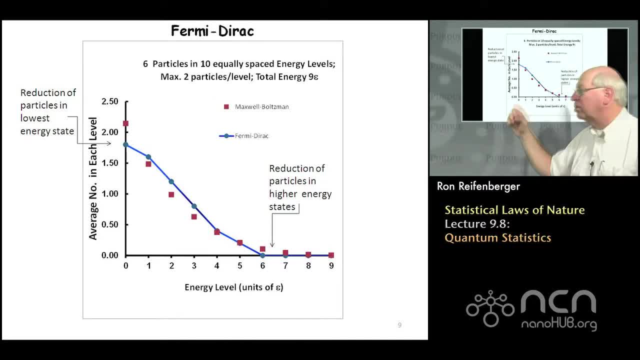 the spin one-half particles. right, that number drops down to about 1.7, 1.8.. And the other important or the other significant difference is that if you look at these higher energy states, there's a noticeable reduction in the number of particles that can exist. 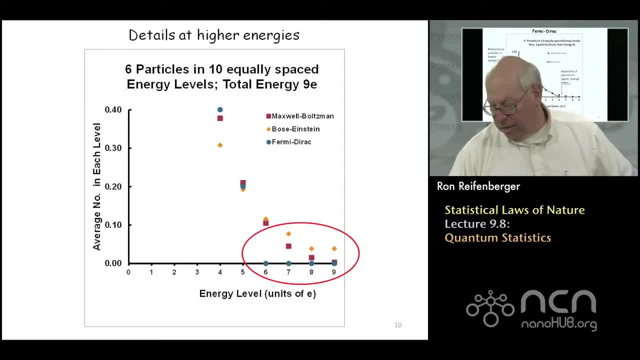 in these higher energy states, And I try to make that point a little bit more clearly here, where I show the comparison now between Maxwell-Boltzmann, the Bose-Einstein and the Fermi-Dirac for these energy levels six, seven. 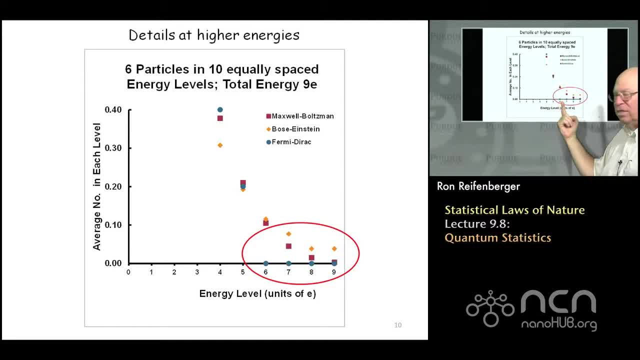 eight and nine. You see that the Fermi-Dirac statistics give you zero particles in these higher energy states, and both the Maxwell-Boltzmann and the Bose-Einstein predicted non-zero values. So there's a significant difference, qualitative difference, not only at the zero energy. 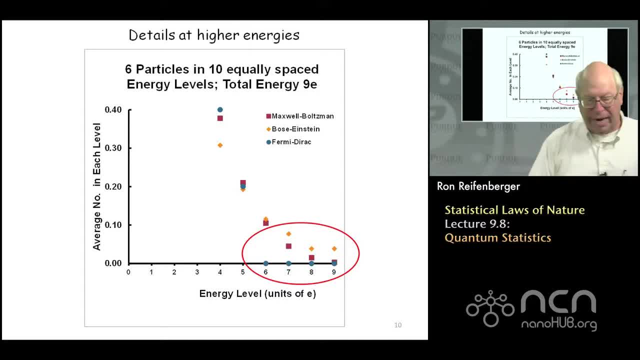 level, but also at the higher energy level for the Fermi-Dirac statistics. And what's amazing is that these subtle differences come out with just six particles in a rather simple system, So they're amplified. these differences are greatly amplified when you start to increase the total number of particles. 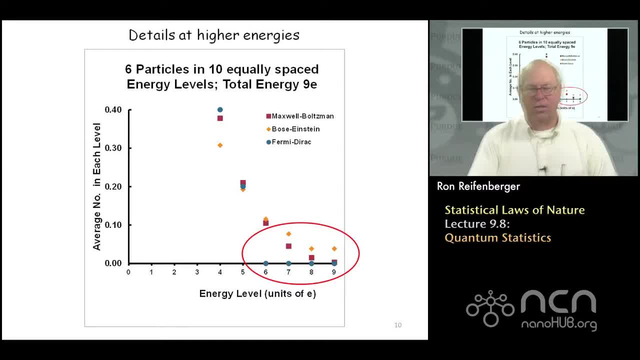 in the system, And what we're going to do next is we're going to derive an analytical formula that describes these probabilities that these various energy levels are populated, And we're going to have different formulas for the classical case. we've already done that, that's. 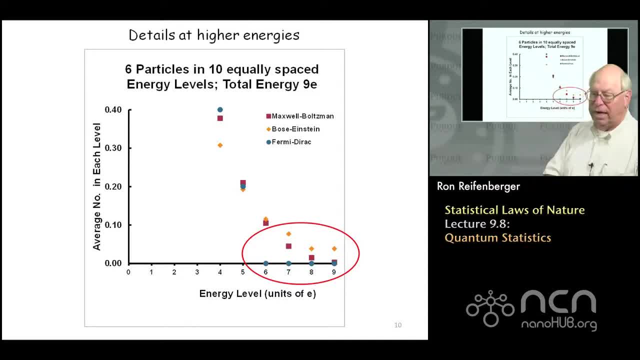 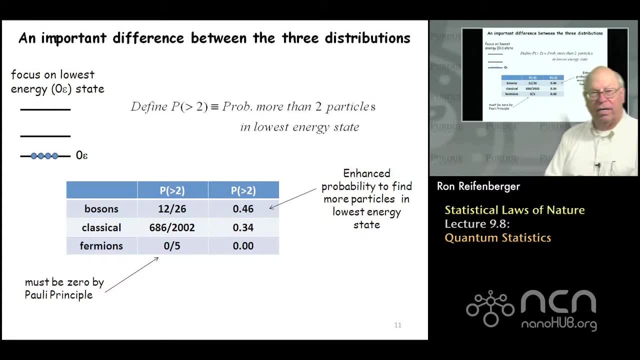 what we're going to do. We're going to write down the formulas for Bose-Einstein and Fermi-Dirac. Let's see. the next slide just makes the case again. I just ask: what's the probability that more than two particles exist in the lowest energy? 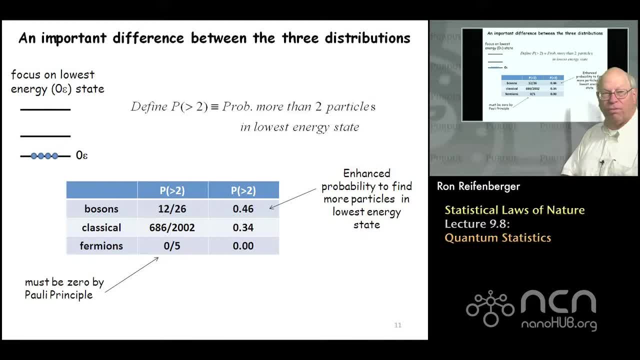 state and I consider the three different types of particles that we were discussing. You can go through the tables and you can calculate. for the classical case, you can find that there's 686 different microstates that have more than two particles in the zero energy level. That's 686 out of. 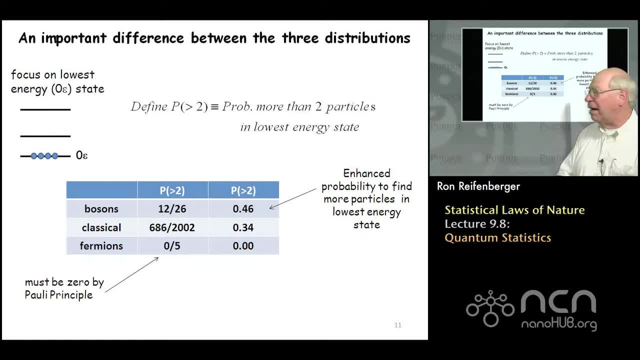 2002, which means that there's about 34% probability that you're going to have more than two particles in that zero energy state. If you do the same calculation, you get about 12 states out of the 26 possible. that gives you 46% of all possible states have. 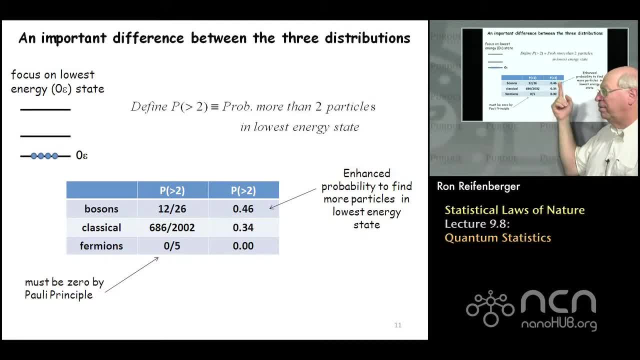 more than two particles in the ground state. so there's an enhancement for the bosons, For the fermions. it's impossible, you can't have more than two particles in any given state. so there's going to be no states that have more than two particles. so for 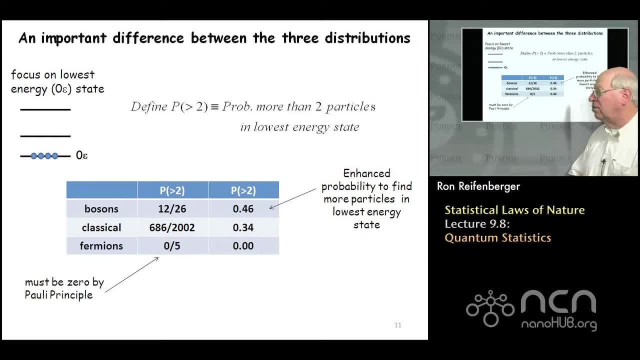 example, the probability that you're going to have more than two particles in that ground state energy is zero. So this again is just another way to reinforce this idea that the type of particle influences the type of statistics. The way that is done is by influencing the number of microstates possible for 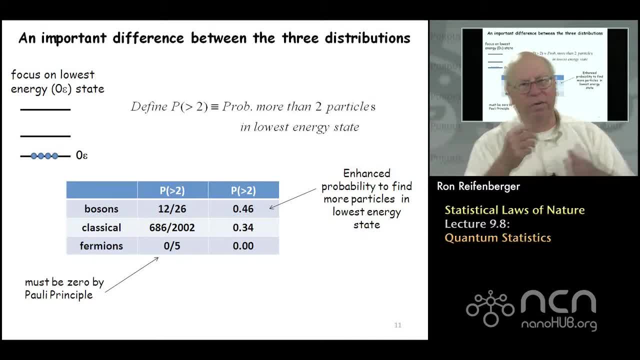 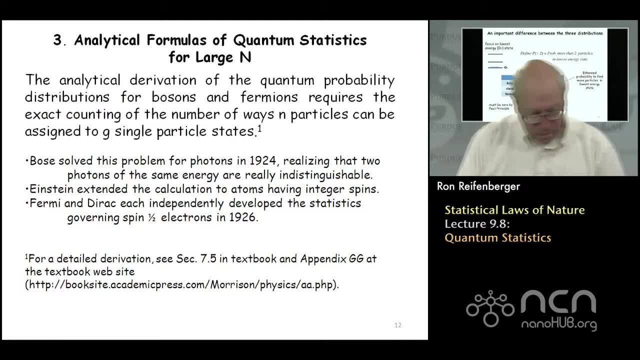 a given system and when you follow that through, even at a very simple level, you start to pick up differences that are significant. So what are the analytical forms for the quantum statistics when you start to let the number of particles get very large, And this is a very complicated? 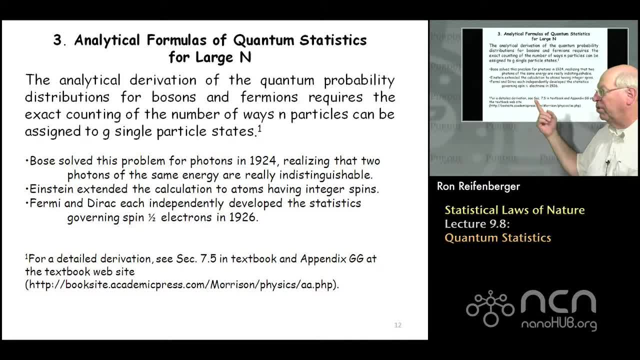 derivation. If you really want to see the details, you can go to the website that I give in the appendix. In the appendix I give some simple arguments that reproduce the derivations in the textbooks. My derivation is a little bit more intuitive. it's: 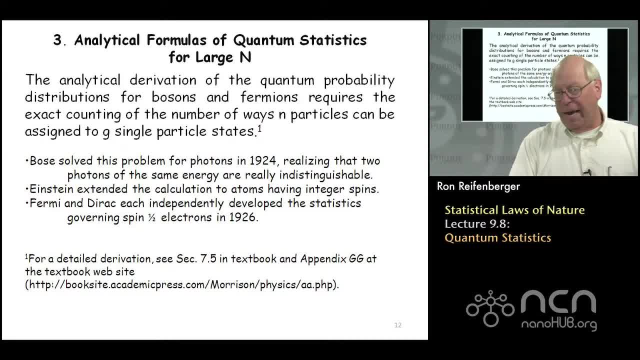 not quite as mathematical as the ones you typically find, and so you have a choice of reading the appendix if you want to understand how these formulas come about, or you can try to sort through the detailed mathematics that you can find in the textbook that we've chosen for this course. You have two. 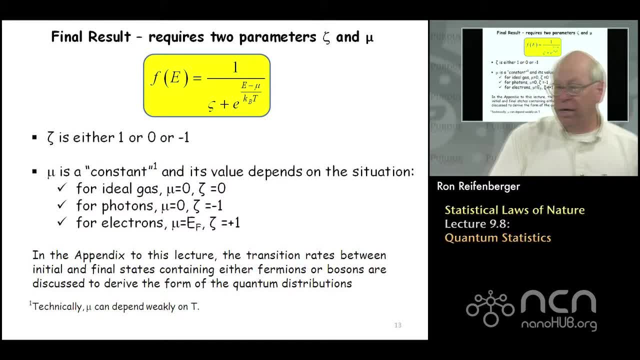 options. Most of you are just going to be interested in the final result, and that's what I quote here. So this parameter f is a function of energy. E is telling you the probability that a particular energy state is occupied in a system, And this 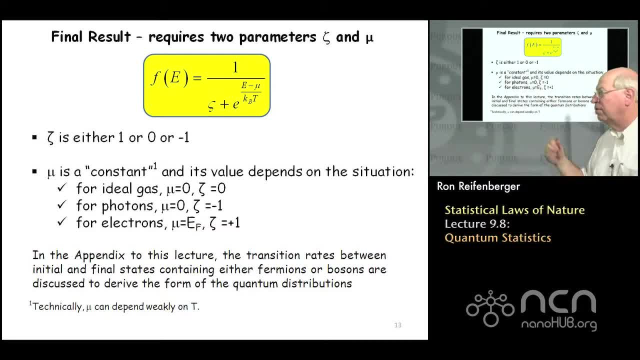 parameter is called mu, And it turns out that probability can be expressed in terms of a universal formula that contains two adjustable constants. One constant is zeta. the other constant is this parameter, mu, And depending on different systems, zeta and mu will have different values. So zeta turns out to 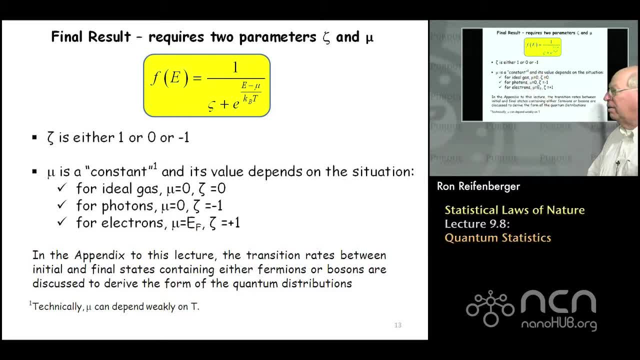 be either minus one zero or plus one, And I'll show you which value of zeta applies to which situation. Mu is a parameter that basically defines the zero of energy of the system, and mu has different values, again, depending on whether you're. 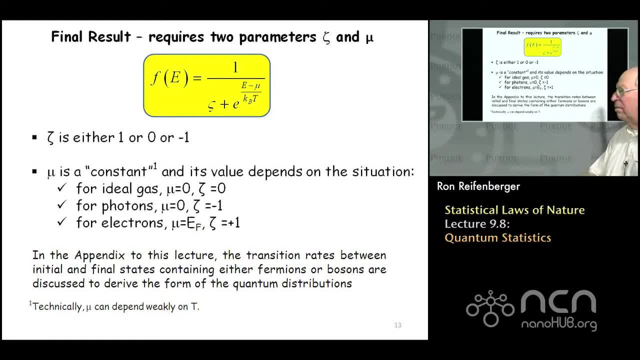 talking about classical gas atoms or photons or electrons. So the appropriate values for mu are different values for zeta and mu, and mu and zeta are listed here for a couple of simple situations And then in the next slide I just 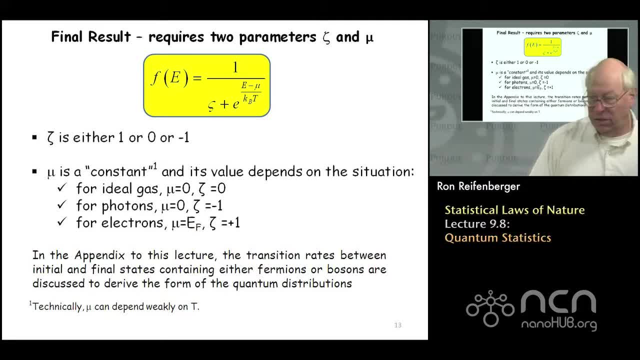 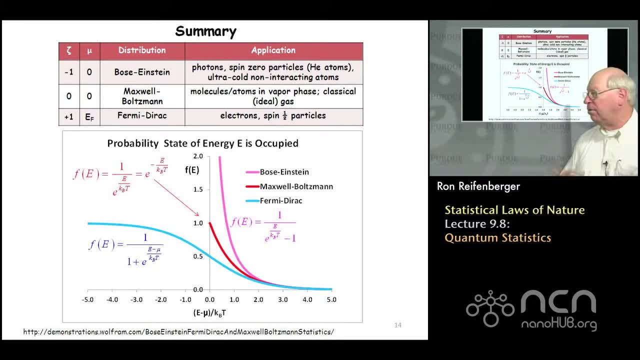 summarize the results in a convenient table and I include a graph so you can visually see what this distribution function f of E is trying to convey. So this is the distribution function f of E is trying to convey. So we've got three situations that we've discussed. 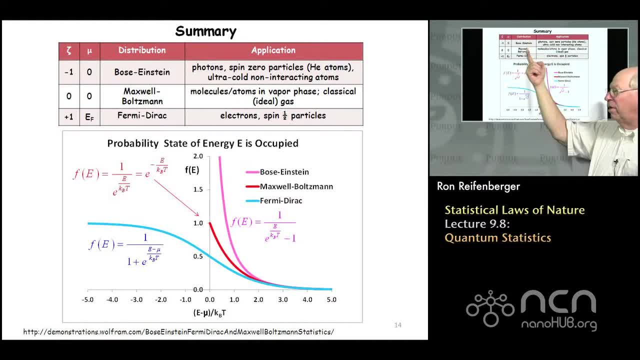 We've discussed the Bose-Einstein particles, we've discussed the classical Maxwell-Boltzmann particles and then we've discussed electrons, which are governed by the Fermi-Dirac statistics And, depending on which system you're interested in, zeta and mu have different values, And what I've 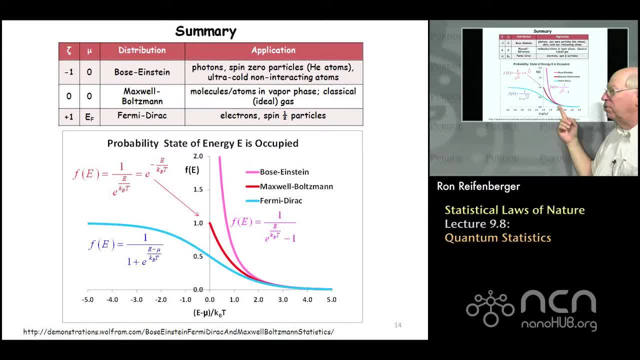 plotted is the shape of these distribution functions for the three different situations. So the simplest one to comprehend is the Maxwell-Boltzmann distribution. This is the exponential decay of particles at higher energies, and that's something that we've discussed in the context of the Maxwell-Boltzmann distribution of 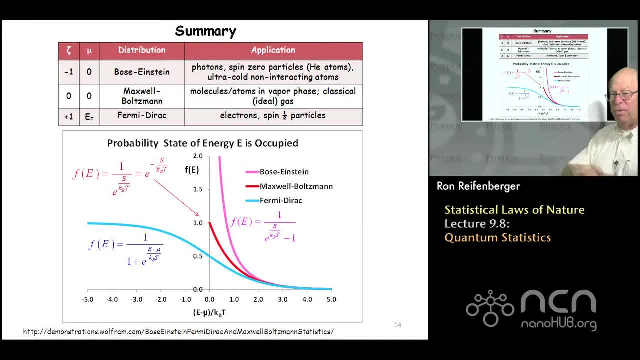 velocities or energies of particles in a classical gas. In contrast to the Maxwell-Boltzmann distribution, the Bose-Einstein distribution essentially agrees at higher energies. but as you get to lower energies you find that the Bose-Einstein distribution shoots up. 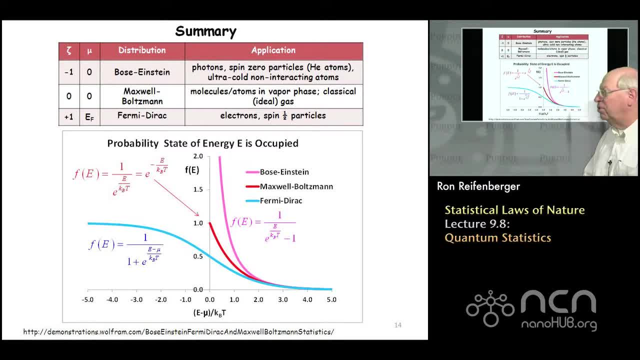 gets very large and significantly deviates from Maxwell-Boltzmann. This is just telling you that, for low energies, if you have a gas of Maxwell-Boltzmann particles, you're going to have a very high energy density. If you have a collection of Bose-Einstein, 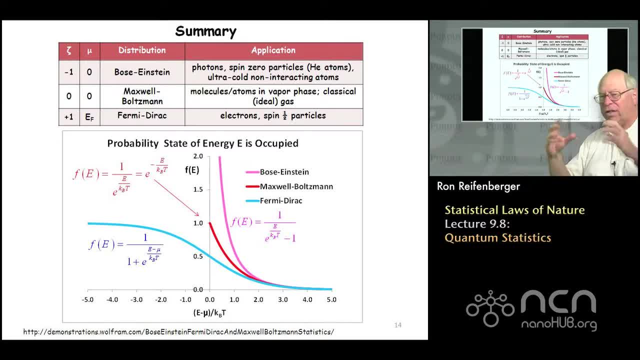 particles, you're going to find an increased tendency for the particles to exist in lower energy states compared to the classical case. When you deal with electrons, with fermions, then you have to use the Fermi-Dirac distribution function, The Fermi-Dirac. 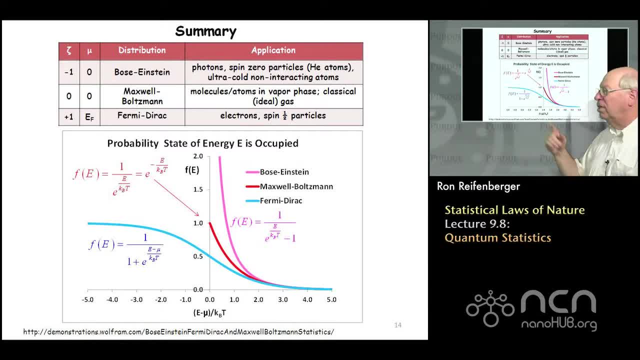 distribution function saturates at unity when you're at energies much lower than this characteristic energy mu and as you go to energies much higher than this characteristic energy mu, it turns out the Fermi-Dirac statistics essentially match those of Maxwell-Boltzmann. 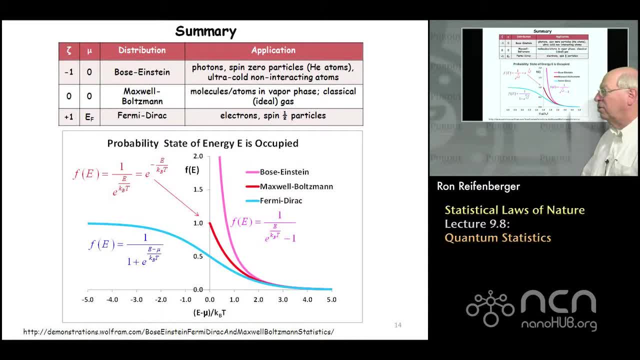 and Bose-Einstein way out here at high energies. In the middle there's a transition from a unit probability. so if you have an energy distribution function from a unit probability, so down here at these lower energies, the states that exist down. 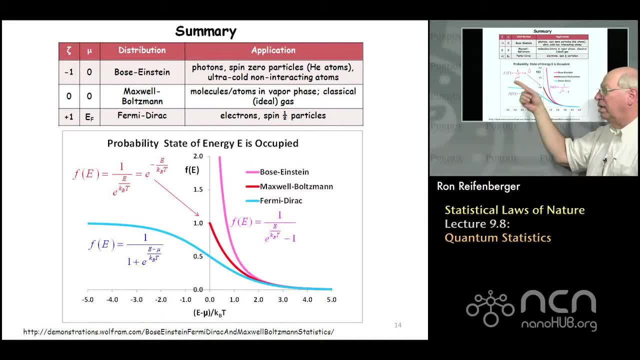 there are populated with unit probability. right at when the energy E is equal to this parameter, mu, the probability of occupation is equal to one half. and then, as you go out to higher energies, when E minus mu is much greater than kT, then the states out there are occupied goes to zero. 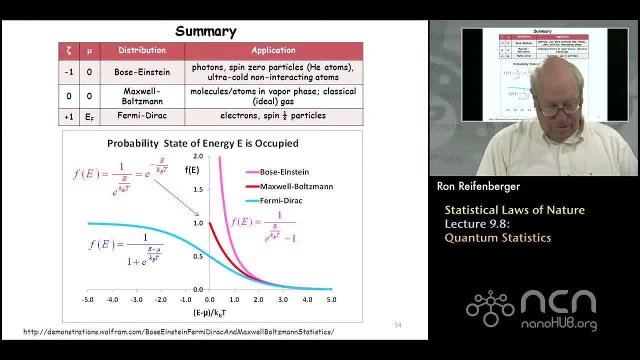 So this is kind of the culmination of our discussion of statistics. A lot of textbooks just give you these results and they don't give you any intuition about where they came from. The approach I've tried to follow is: I've tried to cook up a simple enough system that you can apply these. 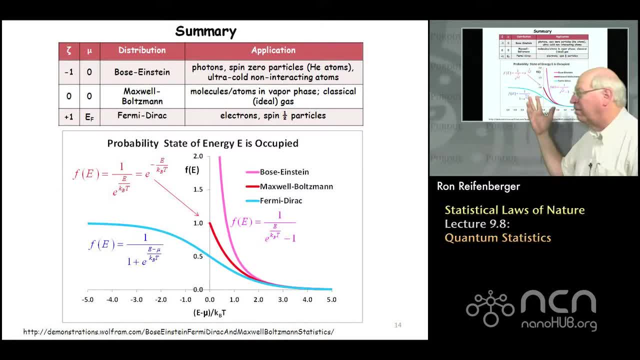 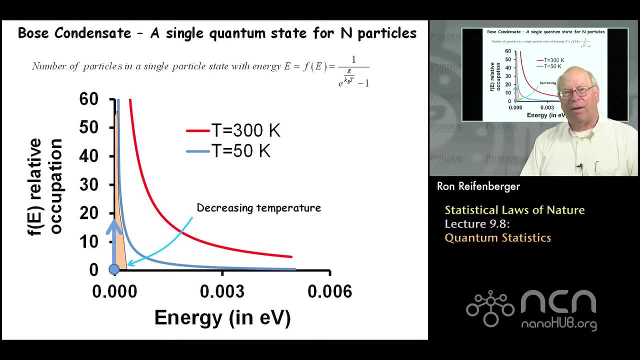 functions and get a much better intuitive understanding of what the fundamental differences are between these three very important distribution functions. I wanted to say a little bit more about the Bose-Einstein distribution because it's been a topic of considerable interest in the literature during the past ten or so years. 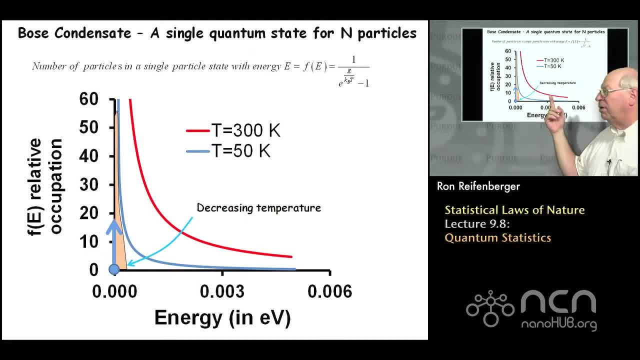 I just want to make the point that if you take the Bose-Einstein distribution function- this is the F of E- and you just plot it as a function of temperature- what you find is that as the temperature decreases, the sharpness of this curve increases dramatically. 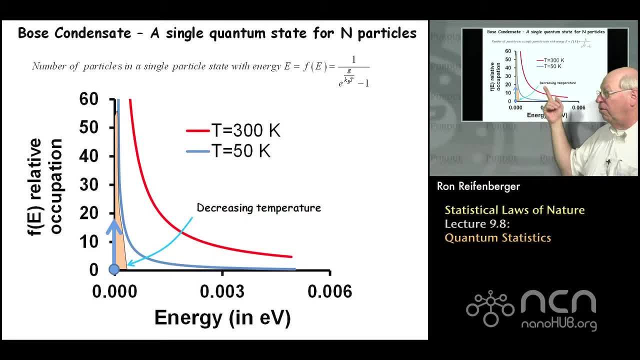 And what this is just telling you is that as you go from, let's say, 300 Kelvin to, let's say, 50 Kelvin, the probability that these higher energy states are actually occupied, that probability gets very, very small And in the limit as t gets smaller and smaller. 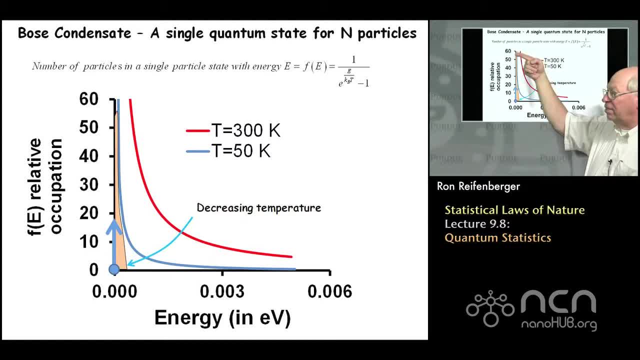 what you find is that this Bose-Einstein distribution function is very, very narrowly peaked around this zero energy level And in fact, what we say is that if you can cool the collection of bosons, so if you have n bosons you can cool. 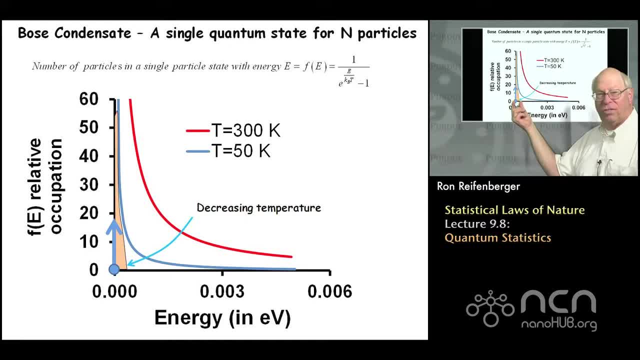 those atoms down to a low enough temperature they actually condense and they form a Bose condensate and all the particles have a very strong tendency to be in one single quantum state. So you've got, let's say, a collection of n bosons and n atoms. 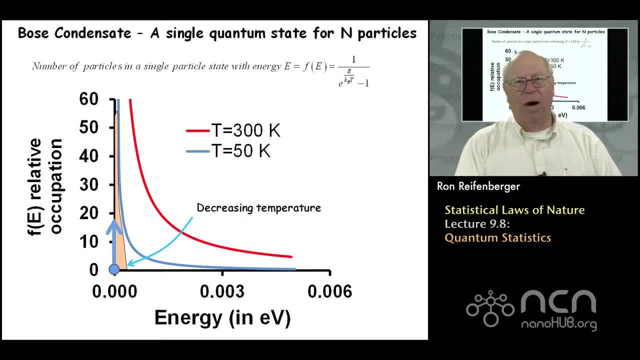 with zero spin. If you cool those atoms down to a low enough temperature, they'll condense into a single quantum state, forms a single quantum state for the entire collection of n atoms. So this has been understood, I think, since the 1930s. The question: 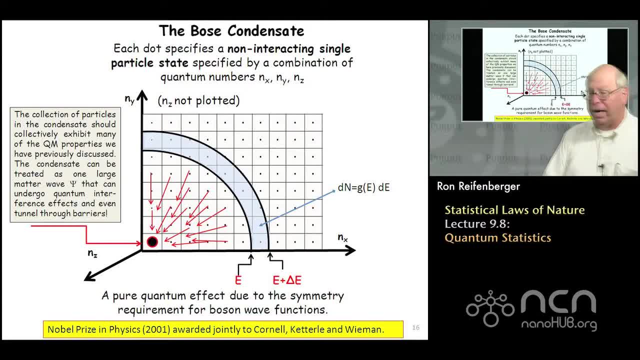 is how to achieve it, and that's proved to be a little bit more difficult. It was finally achieved in the late 1990s. The Nobel Prize in Physics was awarded to the three gentlemen who actually created the Bose condensate And the reason it's interesting. 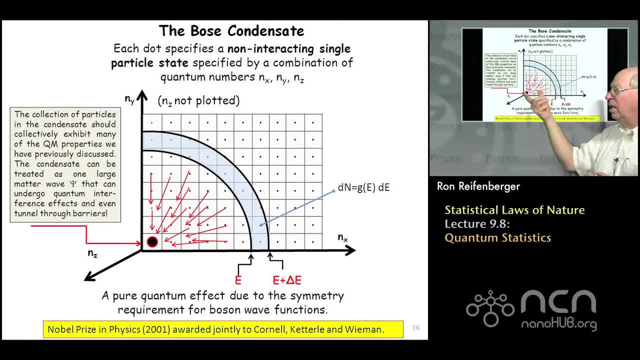 is because, if you go back to our discussion of quantum numbers, for instance of particles in a three dimensional box, each quantum state can be represented by a triad of quantum numbers: nx, ny and z. So each dot in this diagram represents an individual. 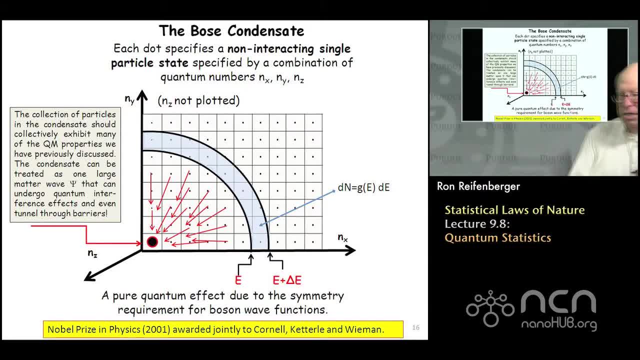 quantum state. What these Bose statistics are telling you is that if you cool this system down to a low enough temperature, all these quantum states condense into this lowest energy state, which is represented by this black dot down here. And this lowest energy state is still a quantum state, but it just has. 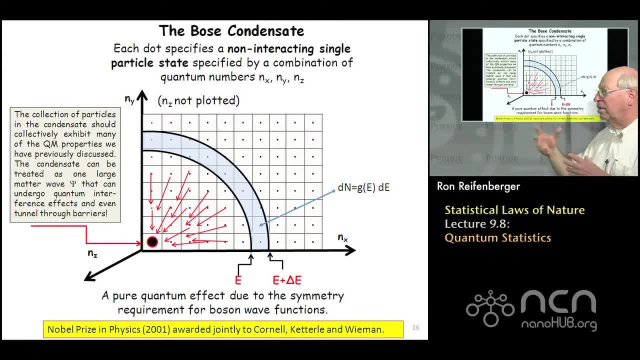 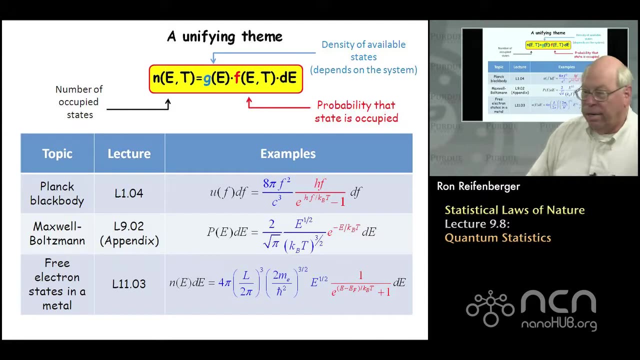 all these other particles that were in these higher energy states present. So there's a huge condensation of these particles into one massive quantum state which has very interesting physical properties, and that's a topic of intense interest in the physics community even as we speak. So by way of summary, 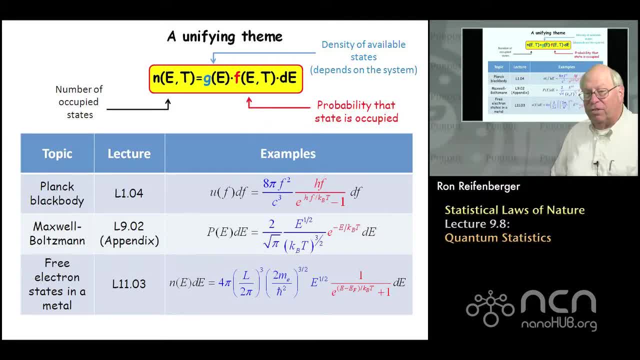 I wanted to just emphasize a unifying theme that I hope will tie together some of the lectures that I've given in the last couple weeks, And this unifying theme is the calculation of the number of occupied states in a given quantum system, And this number. 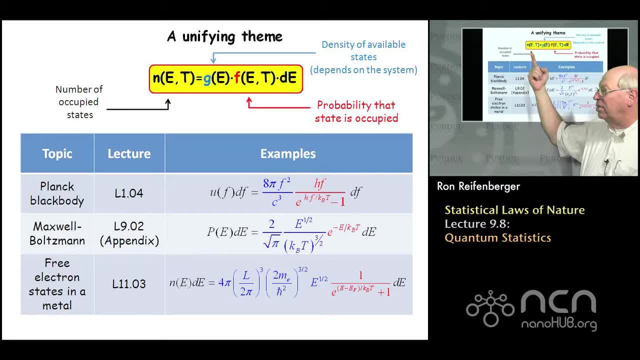 of occupied states is basically related to the density of available states, and the density of available states I've used the symbol g throughout these lectures to represent. So g depends on the particular system that you're interested in. The system does not have to be a quantum system, it could be a classical. 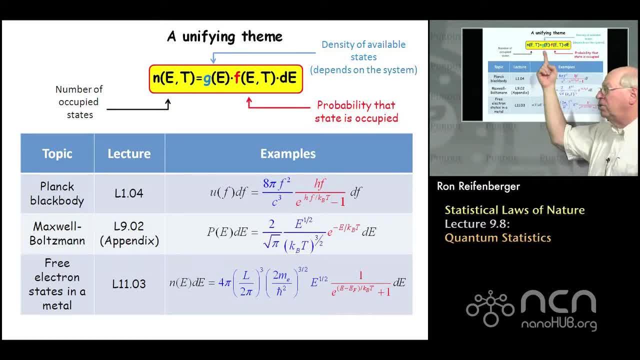 system. But each system that you consider is going to have a different density of states, and you need to know that in order to calculate how many of those states are actually occupied, In addition to knowing the density of available states, you've got to know the 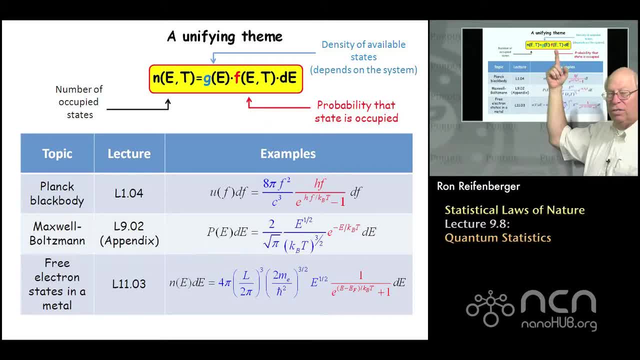 probability that each state is occupied and the probability of occupation is given by this function f. And this function f, there's only three choices for it. It can be either a Bose-Einstein distribution, it can be a classical Maxwell-Boltzmann distribution or it can be. 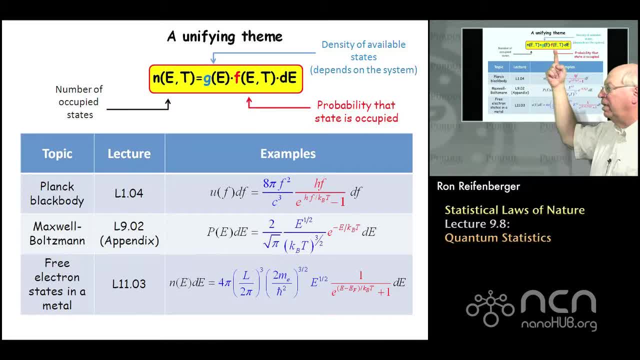 a Fermi-Dirac distribution. So f describes the probability that a state is occupied. g tells you how many states there are. if you multiply these two things together and multiply by an energy interval, delta, E- that tells you how many states of that particular energy are occupied. 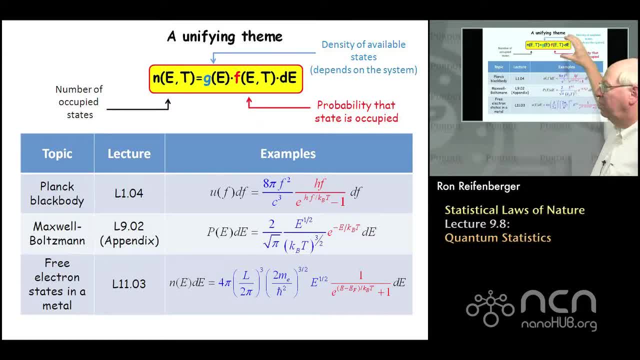 within this energy interval, delta E. So this formula, which I think I included in the first slide, maybe two weeks back, this formula is the unifying theme that sort of links together all these discussions that we've had. We've had discussions that consider both. 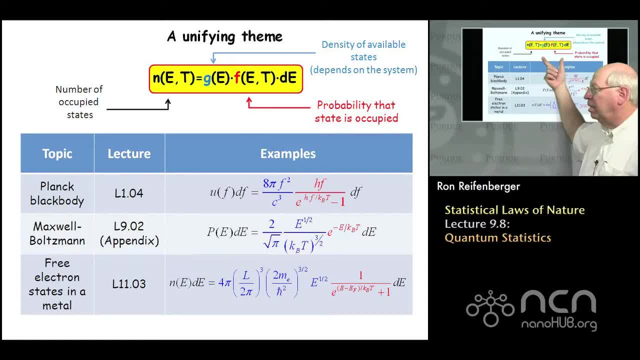 these quantities separately. but the payoff is that when you combine them in this way, you can actually start to tell something about the number of particles in different energy levels for different systems of interest. And just to sort of reinforce that notion, if you go back and you look at my lecture notes, there's 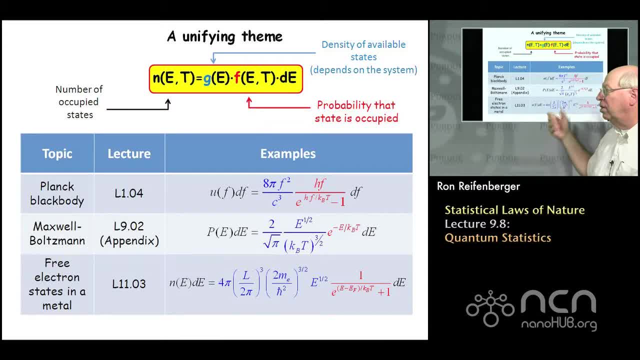 at least three separate occasions where we've written down results, and these results can be understood in terms of this unifying theme. If you recall, back in the first week of the course, we talked about the Planck's blackbody density of radiation field. Well, it turns out. 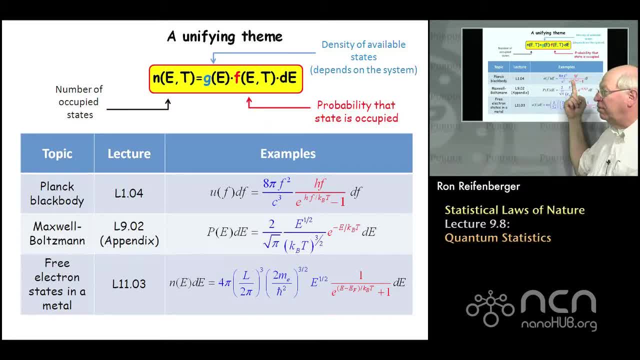 if you write that formula down, this pre-factor here is telling you something about the density of the photon states and this factor here is telling you about the occupation probability of those states. So this is the Bose-Einstein distribution function which we now. 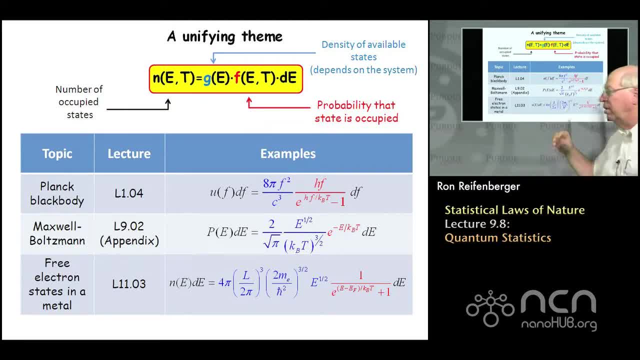 appreciate, but which Planck didn't have a clue of back in 1900 when he worked this out. If you go back and look at the Maxwell-Boltzmann distribution function that I have to look at lecture 9.02, if you. 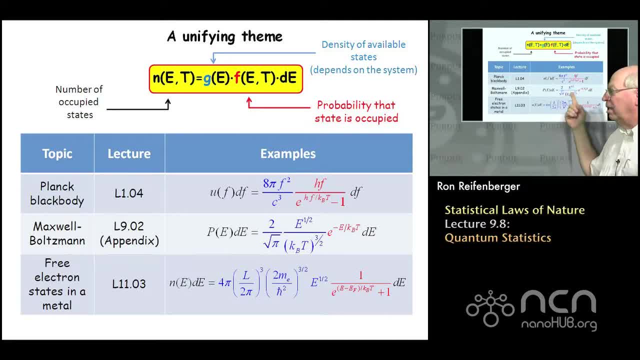 look at the appendix of that. this exponential factor here is the Maxwell-Boltzmann distribution. that's the probability, the state of given energy. E is occupied. This pre-factor here is basically a density of states term which tells you how many atom states. 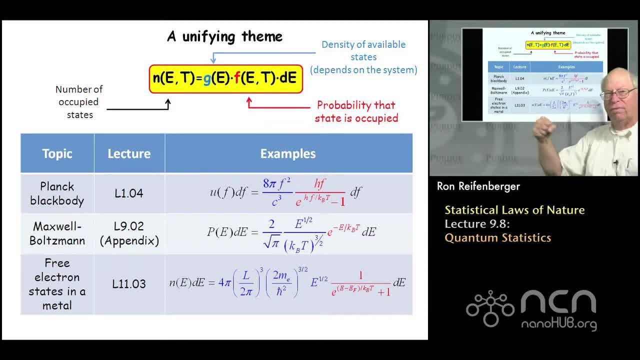 are available? how many molecule states of a particle moving in three dimensions are available as a function of energy E? And then, lastly, in another week or so, we'll do the case of free electrons and we'll come up with a formula that looks like this: